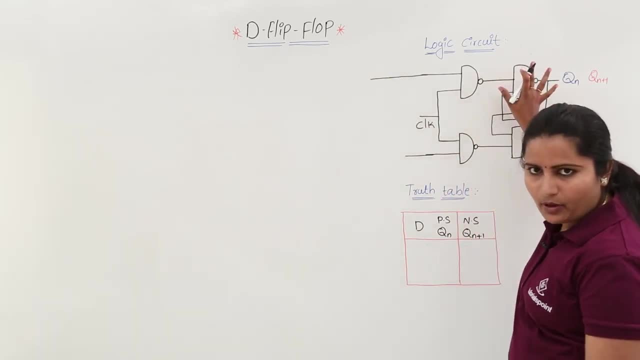 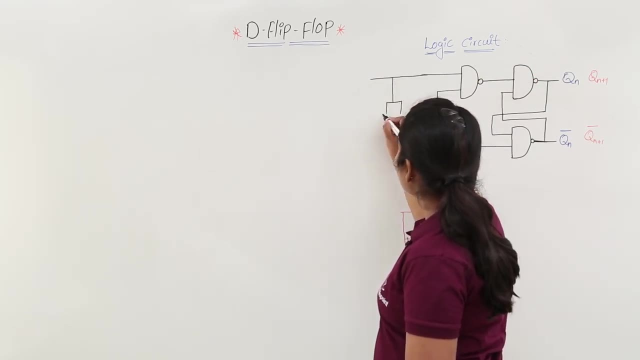 NOT gate in between S and R. you know this is SR flip-flop. So now I am just taking a NOT gate that NOT in the form of NAND. So I am just clubbing two inputs of NAND, it will access NOT gate. So I am just taking NOT gate in between this S and R and I am making this. 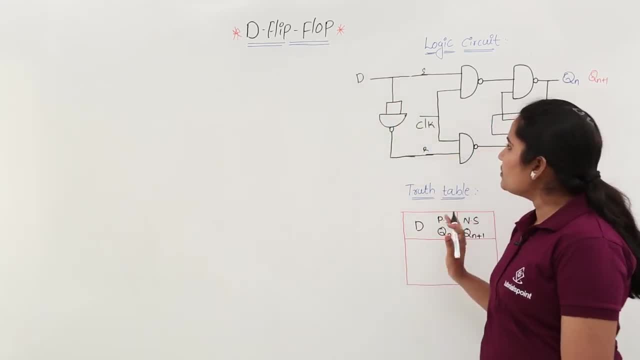 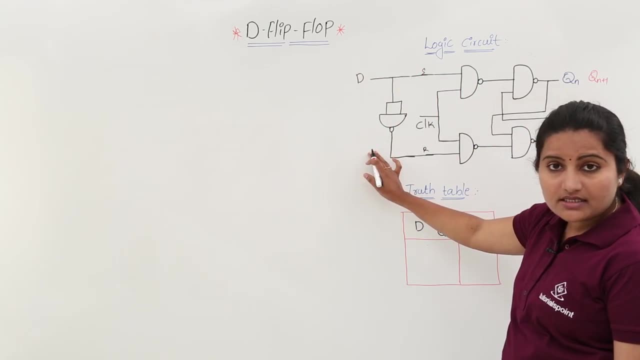 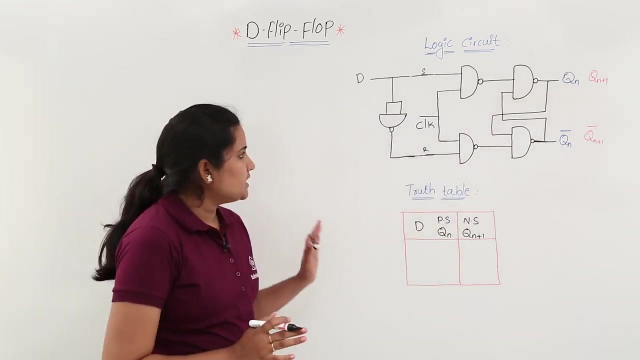 as data line, my data line. So here you can observe: now, D is given directly, that is nothing, but D is equal to S and D is equivalent to R, equivalent to D bar. So now, here I am going to deal the same thing, So which I done previously for SR flip-flop, that is So to. 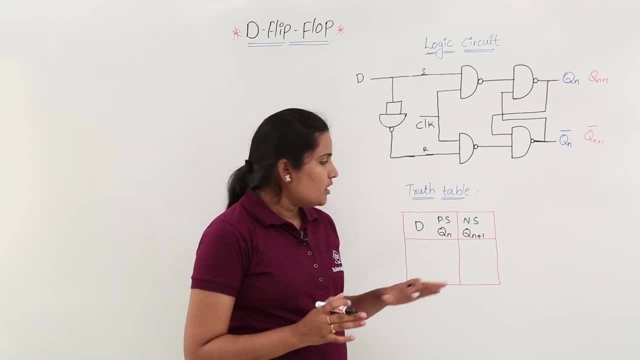 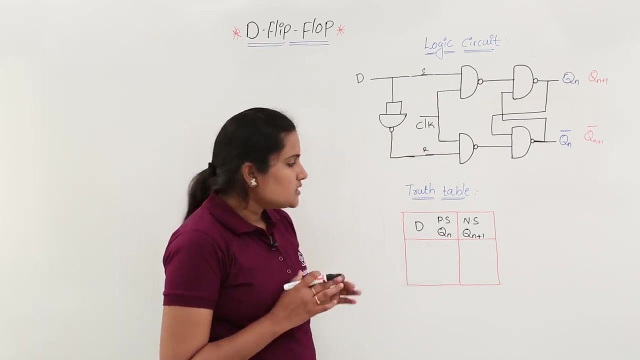 get the expression or to see the operation. we need to take truth table for any sequential circuit, not only for this flip-flops. for any sequential circuit, after having circuit diagram or logic diagram, you need to consider truth table to observe the functionality. So now you can see only one input. So another input may be your present state because to 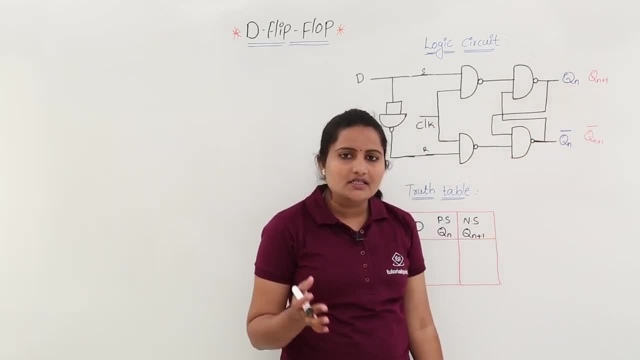 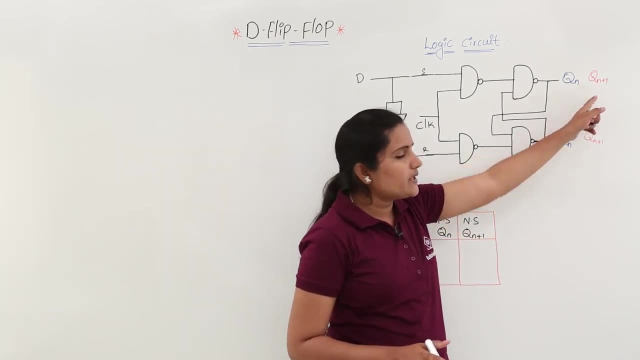 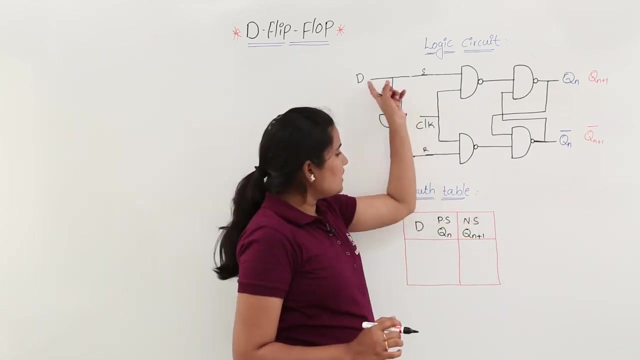 get your output. that means next state. I always telling you that your next state is your output. Next state is your required output for any sequential circuit. that means Q, N plus 1 is your output. What are the inputs for this sequential circuit means? So, actual inputs. 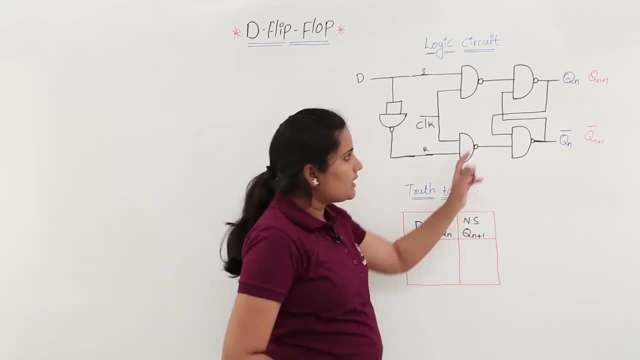 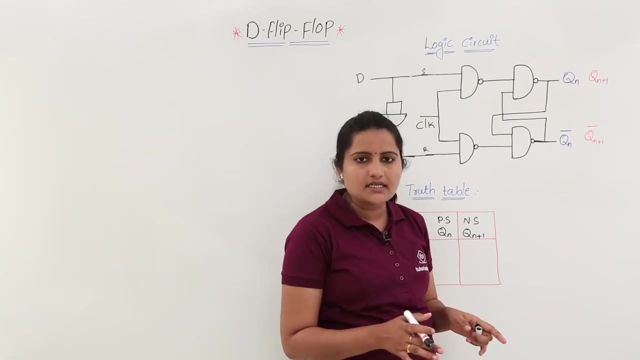 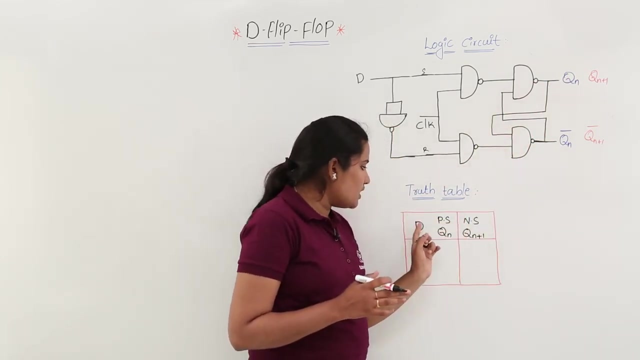 whatever you are observing at input side, those are inputs and present states. whatever state that is in this time, the mission is in this time- that is called as present state. that present state we are giving as feedback input. you can observe like this: So Q R- inputs- here that means data input- and Q N- present state inputs are inputs and 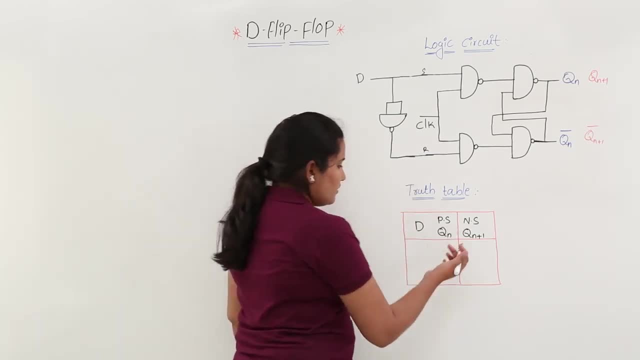 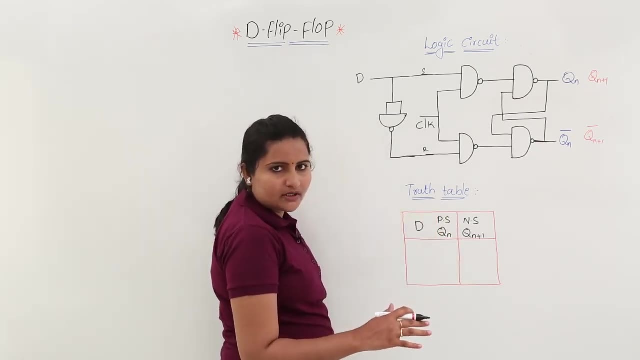 output is next state. So now here I always telling you that here, I already told you that. So always present state. we do not know about this. the present state may be either 0 or 1, we do not know about this. that is why I am taking: do not care of this present state. 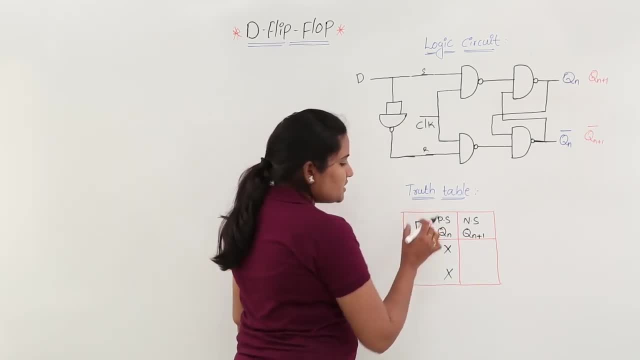 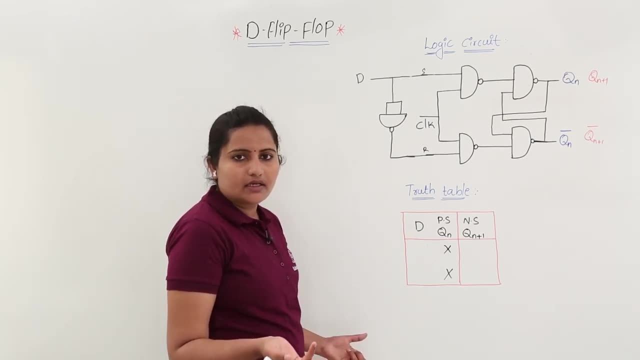 that may be either 0 or 1.. So here the combination of data we can give. as this is a single variable, the data we may give in 0 or 1 data input may be either 0 or 1.. For example, if you are having two input variables, like S and R, you can give combination. 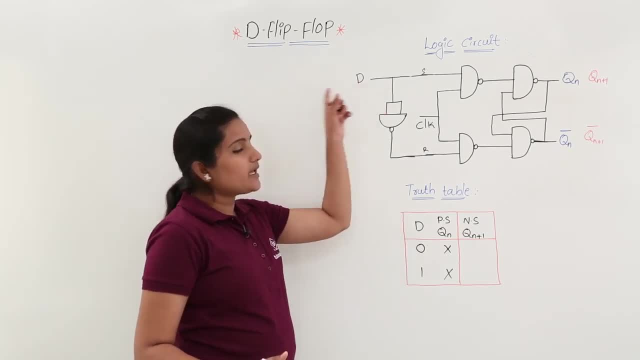 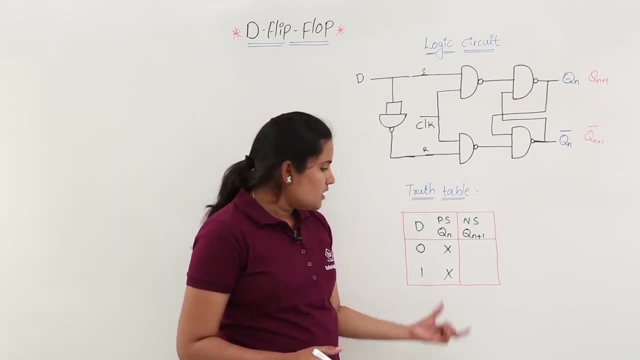 of 4, 0, 0, 0, 1, like that, but here the input line, make that only one line with one variable. we may have only two combinations. that means either 0 or 1.. So now, here I am going to. 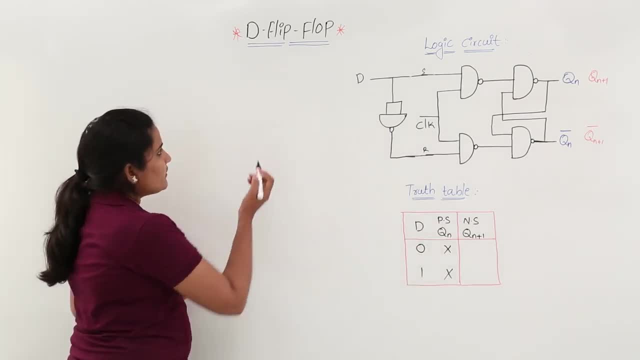 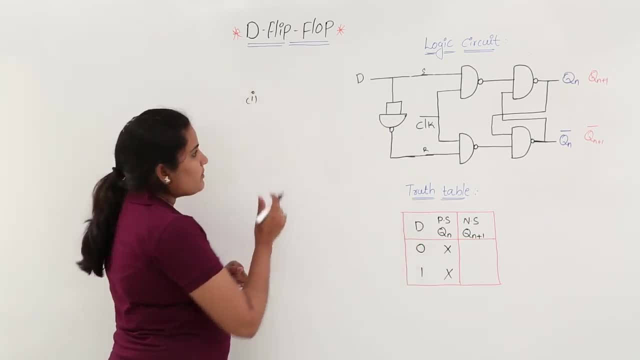 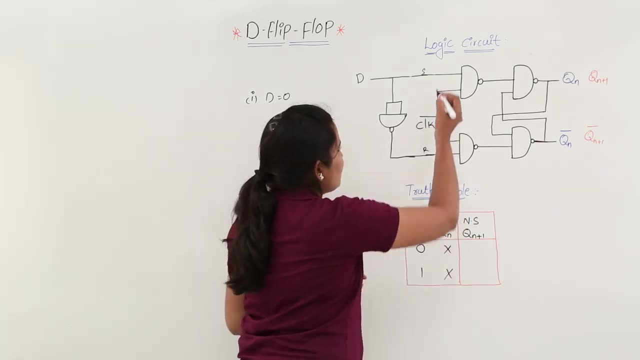 So first case, your first case, is equal to. so D equal to 0 case and considering D equal to 0. If D is equal to 0, the input for this gate is equal into 0. And here you are getting, as you are having not gate, here you are getting. 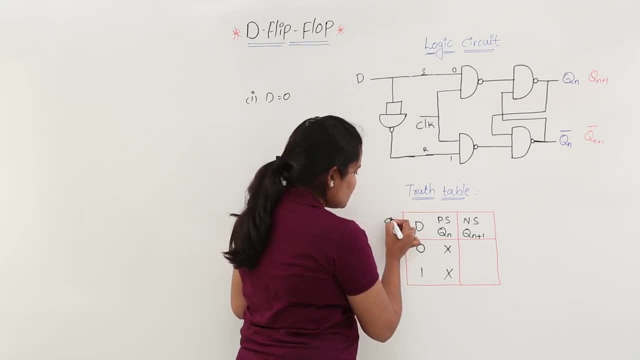 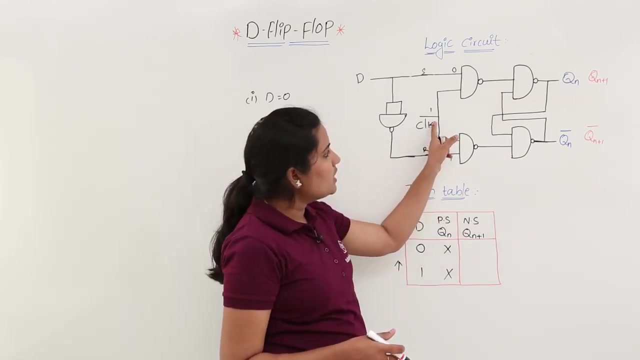 1 here. So always clock pulse. you can consider like clock is on, that means clock is 1. always need to consider clock is 1.. Otherwise your circuit will be in the same condition. you can check if clock is equivalent to 0. definitely you are getting without knowing other input values. 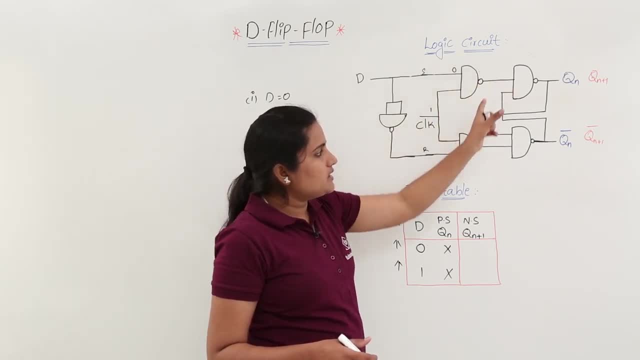 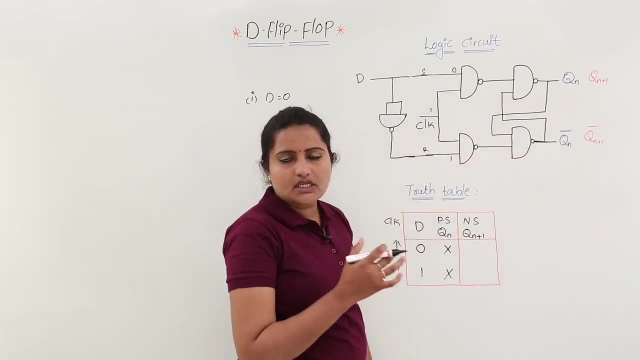 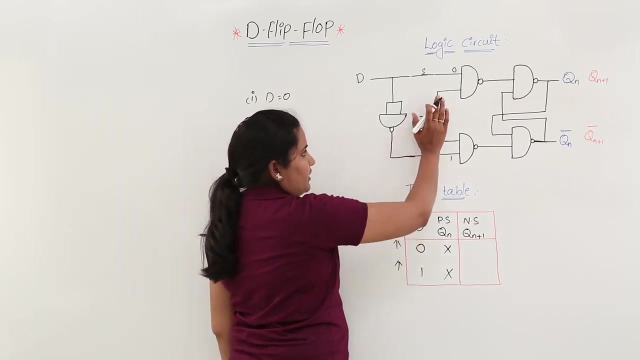 without knowing the input data, your gates, these gates output goes to 1- 1. when it gives 1- 1, your circuit is going to no change condition. So now see here: so always you are taking clock as on. So here, when you have, clock is equivalent to 1, and when you are having your data as 0, your 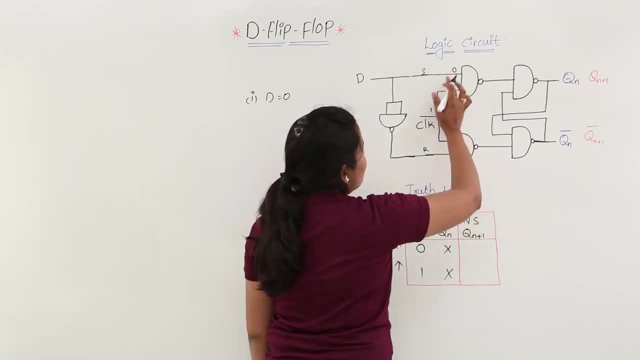 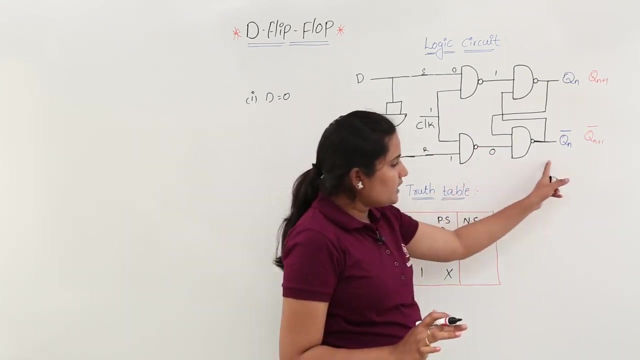 circuit having inputs like this. So now, 0 into 1 whole bar. you are getting 1 here and here, 0. here you are having 1 into 1 whole bar, you are getting 0 here. So now which gate you need to? 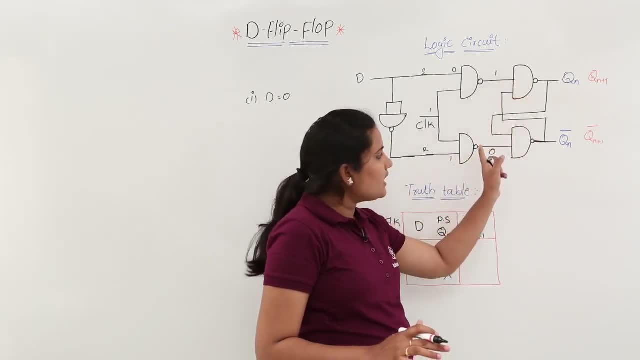 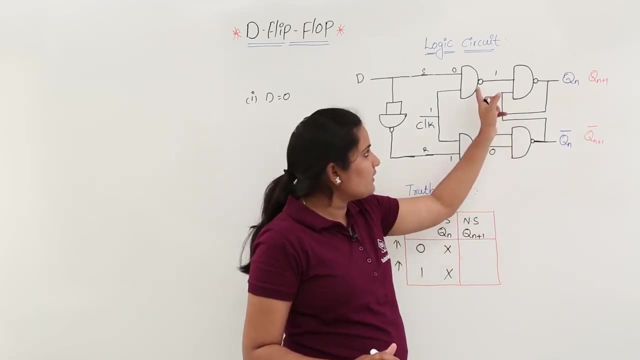 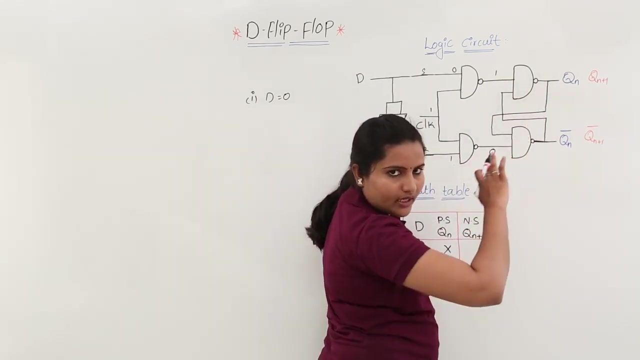 process means: see here as these are nanded. I think it is better to propagate first like this and after like this, because here you are getting value, with that value you are going to get this value. So here, 0 into anything, that means q n, 0 into q n bar is equivalent to 1. here, This one, I am propagating like this, 1 into 1. 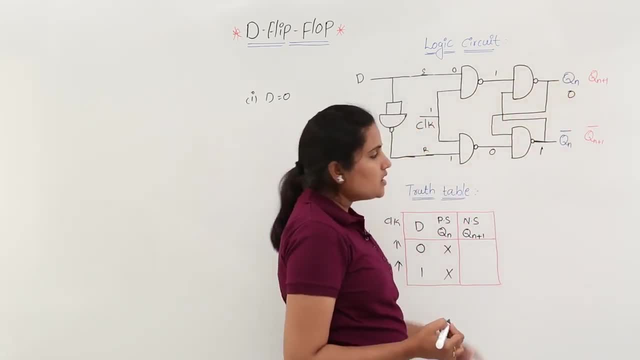 whole bar. you are getting 0.. So 1 into q n, q n plus 1 bar you are having here. So 1 into 1 whole bar, you are getting 0.. So 1 into q n, q n plus 1 bar you are having here So. 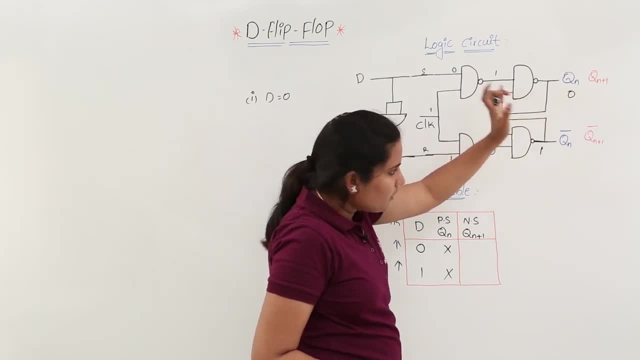 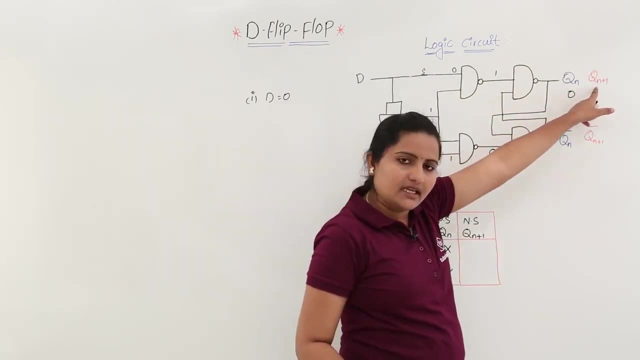 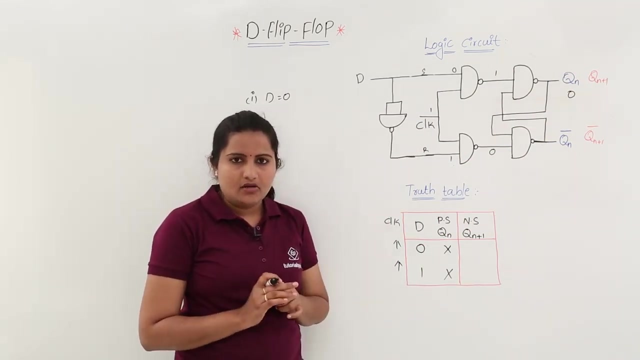 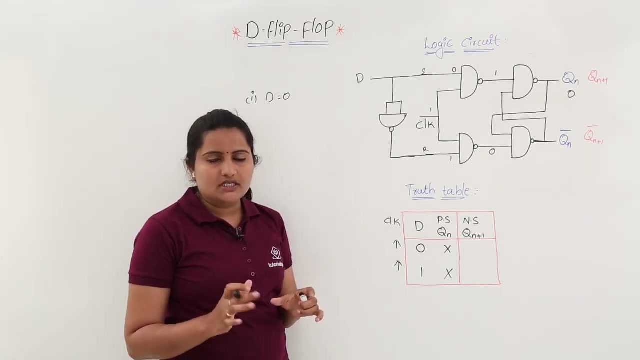 that one I am propagating to top side. or if you are having any doubt like this, So you just propagate your normal line. that means you just take equation for q, n plus 1.. So every time to make clarity or to design any sequential circuit, just follow only one procedure. 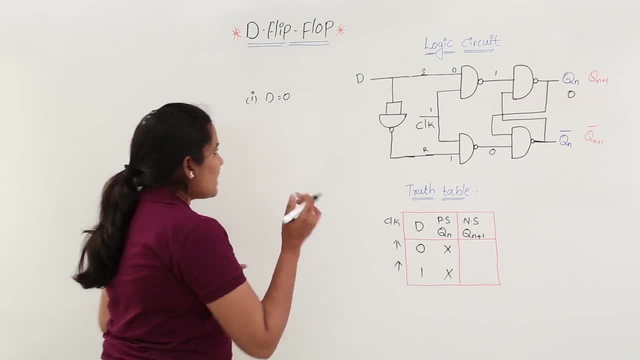 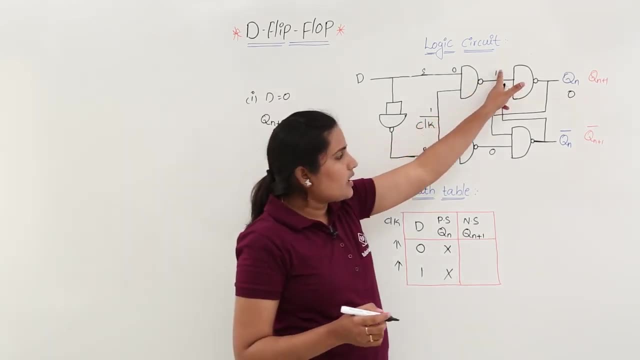 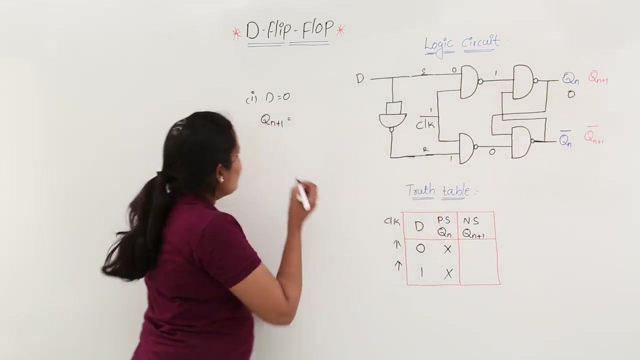 Finally, you need only next state, that is it. So I am just taking when d equal to 0 my next state. I am writing like this: I am taking up to: here: I process q n plus 1 equal to 1 into q n bar whole bar. 1 into q n bar whole bar. this is nothing but q n. 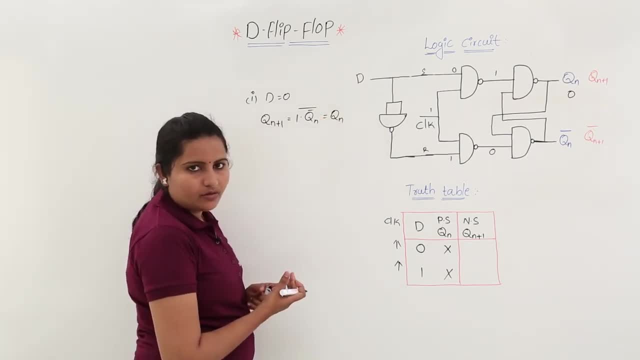 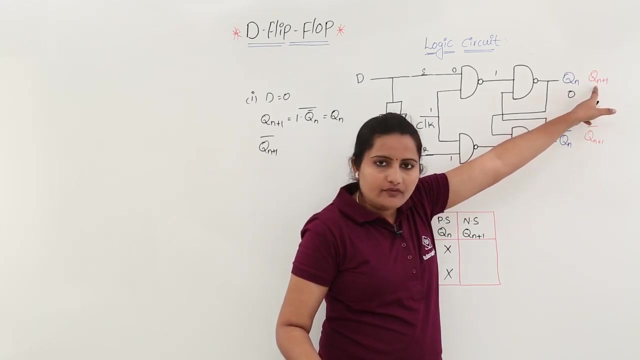 Now, by seeing itself, we cannot say what is the q n value, Then we are going to complement port. If value is available here, either 0 or 1, no need to go for complement. That means q n plus 1 port this port. If here you got value, no need to go for this port. 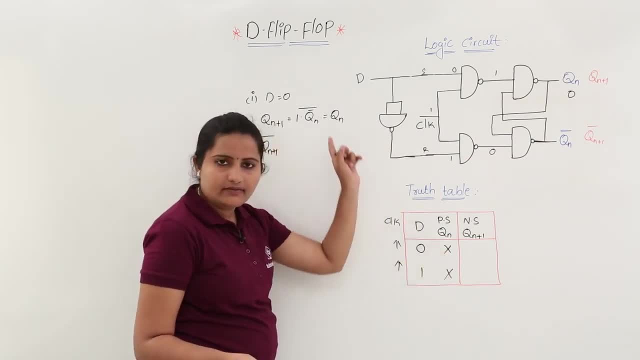 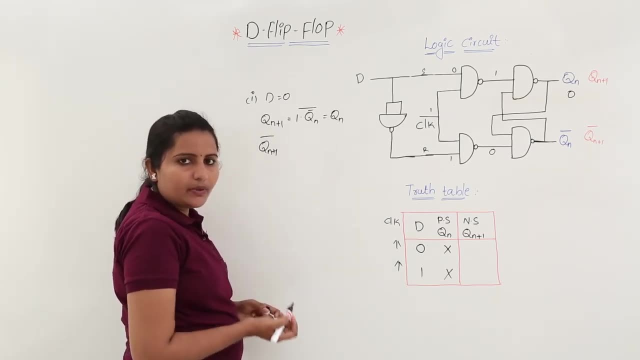 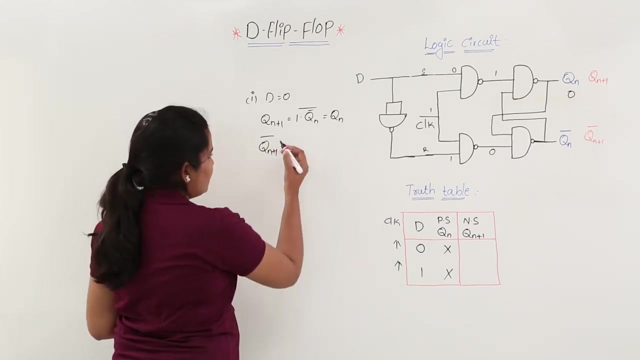 but here you got some unknown value. we do not know that value. So that is why, to get clarity about that value, you are just checking your complement port. If you got value in complement port, then you you can apply that reference to normal port value. that means: So here this is. 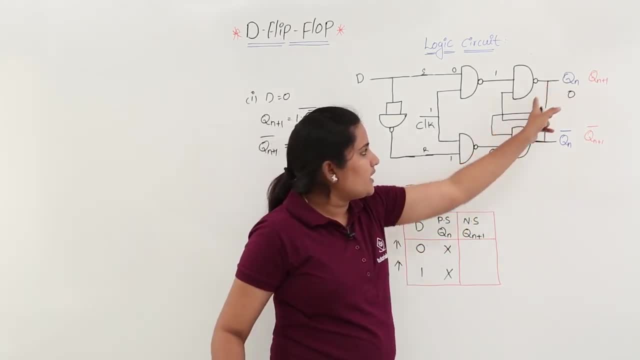 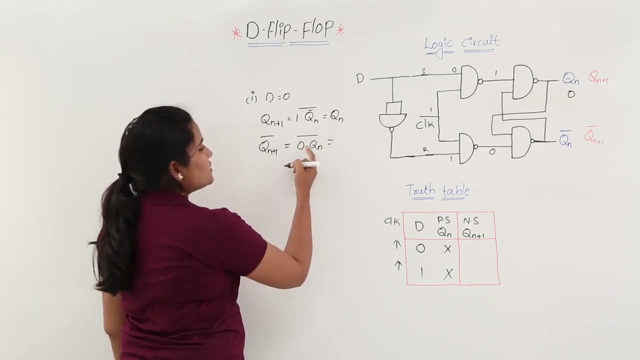 equal to 0.. So that is why, to get clarity about that value, you are just checking your complement port: So 0 into q n whole bar, So 0 into q n whole bar. So here you are getting 0 into anything. 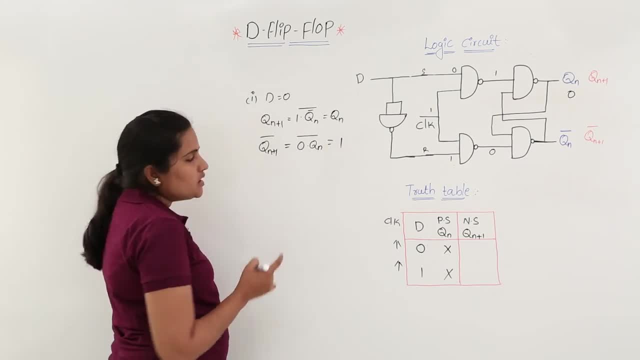 0 whole bar means 1.. So if you got q n plus 1 whole bar is equal to 1, definitely we can reflect this result here. If q n plus 1 bar is equal to 1, automatically q n plus 1 value. 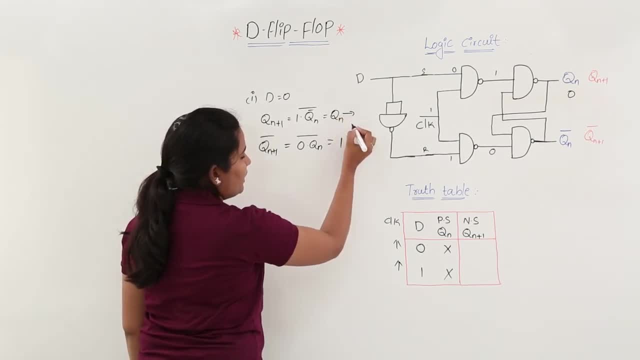 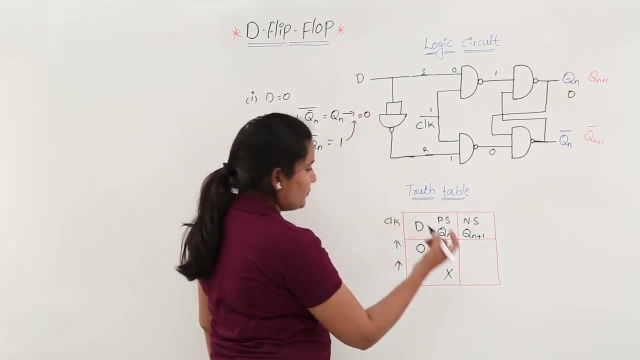 may be 0. So that is why, to get clarity about that value, you are just checking your complement port. So that means, whatever this unknown q n value is there, because of this this is equivalent to 0.. That means your q n plus 1 output is equivalent to 0 in this condition. 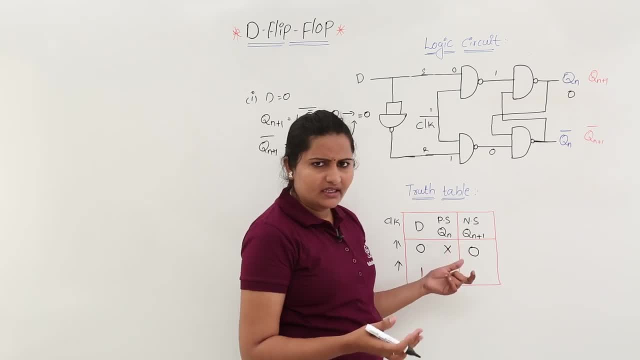 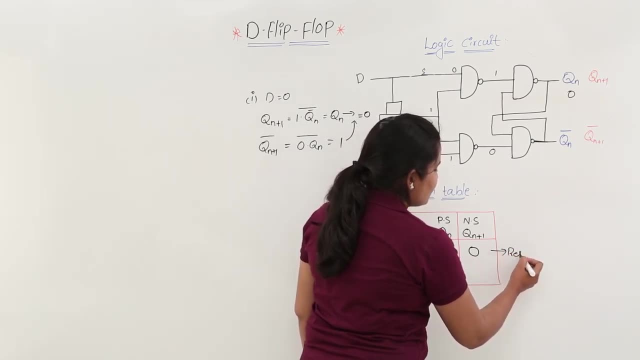 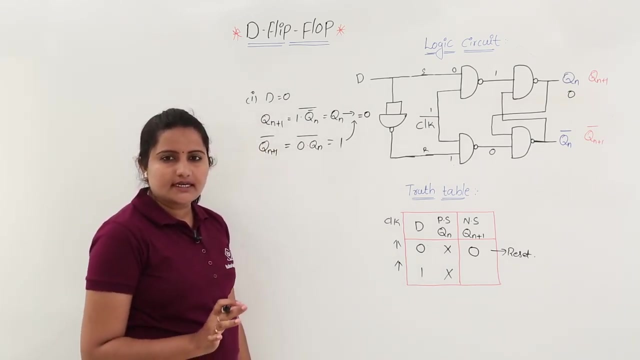 So, without having idea about q n, q n may be anything- your value will goes to 0. So here this is called as reset state. reset state D- flip flop is only having 2 states. So reset state is only having 2 time cycles. So second case is d is equal to 1 case In this q n plus. 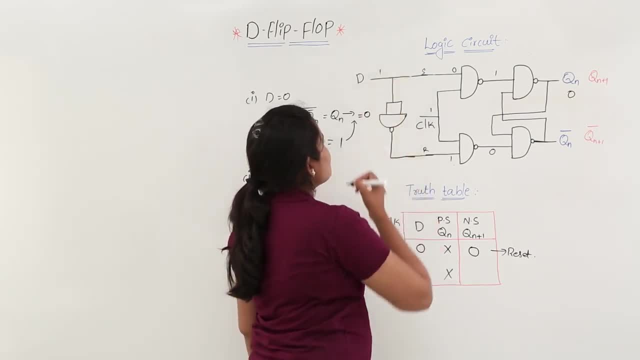 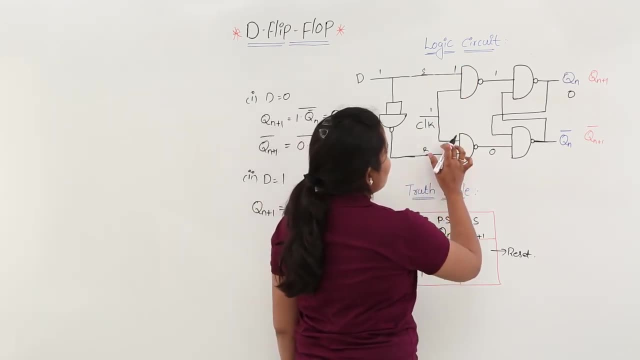 1 you need to define. So if d is equal to 1, that same 1 coming here and 0 coming here. So now 0 into club whole bar- you are getting 1 here, and 1 into 1 whole bar you are getting. 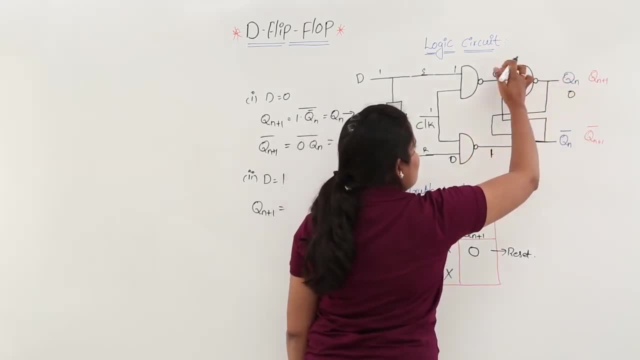 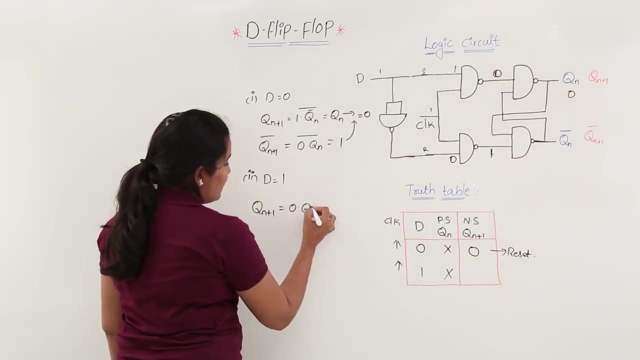 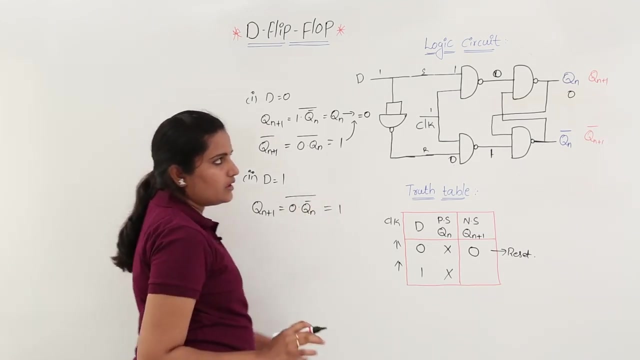 0. here q n plus 1 is equal to 0 into q n bar, whole bar. So I am writing 0 into q n bar, whole bar. here you are getting directly. So 0 bar means 1.. You got value in q n plus 1 whatever you needed for. 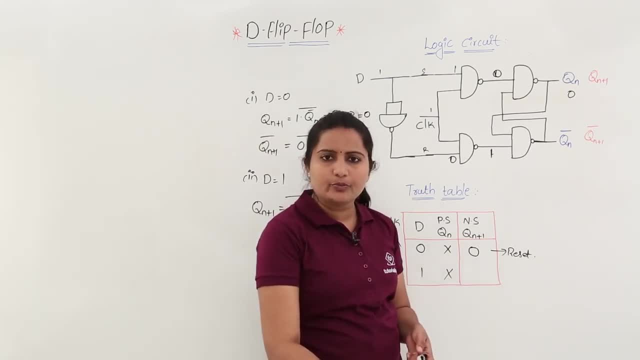 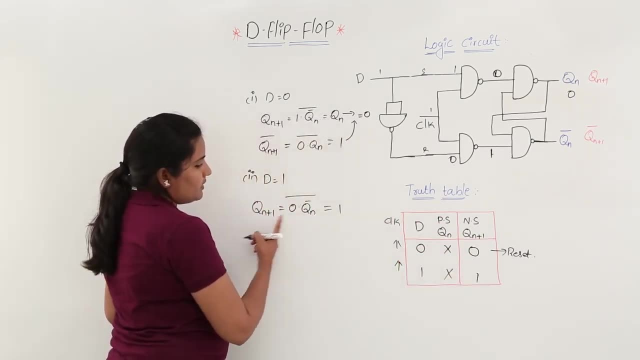 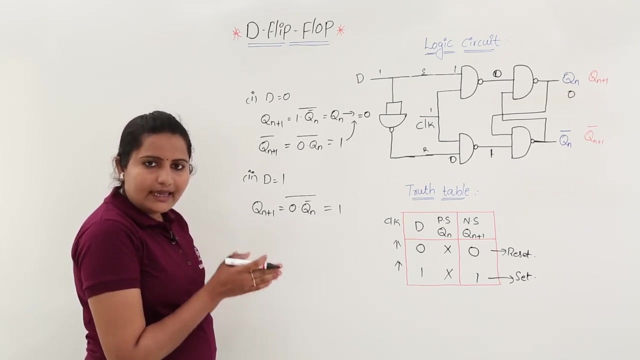 that you got value directly, Then no need to go for complement port and get reference from that. So here you can write when d equal to 1, q, n plus 1 is equivalent to 1.. So you got set state. Now I want to take, I want to draw my block diagram, or I want to take expression for d. 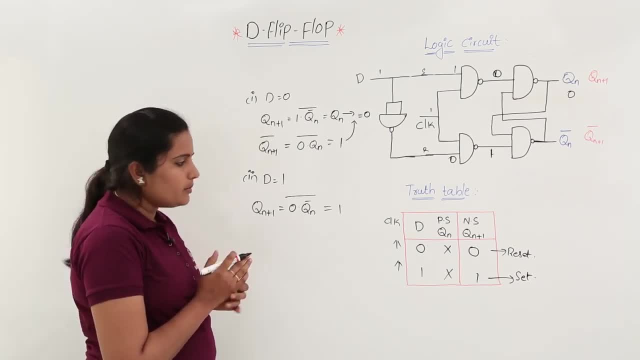 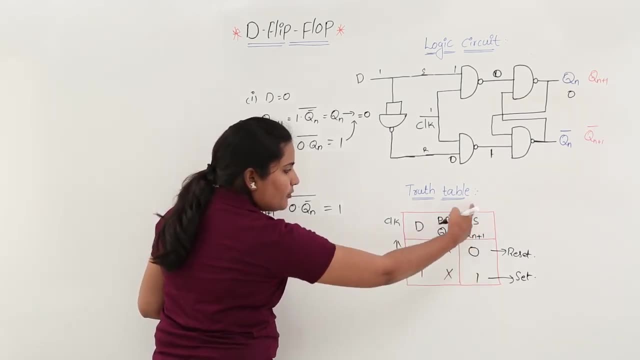 flip-flop To get expression for d flip-flop. So I am just taking k map. How many variable k map we need to consider means Whatever output functionality is there, that is the source of expression. So for this, the 2. 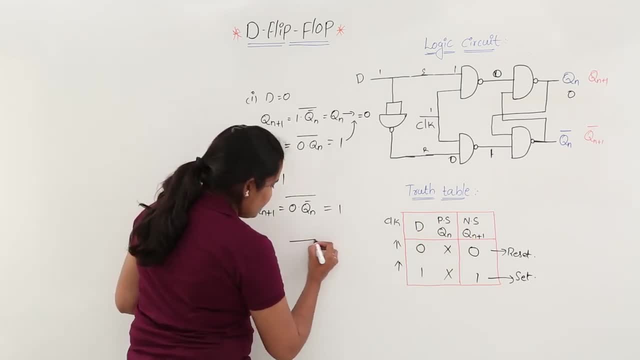 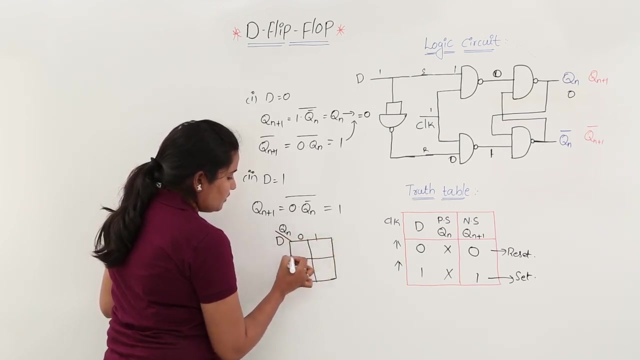 input variables are d and q n. So 2 variable k map you need to consider to get the expression. So I am considering 2 variable k map in that one is input variable d and other is your present state, q n. So I am taking combination with 0- 1 and you are getting, when you are having 1, 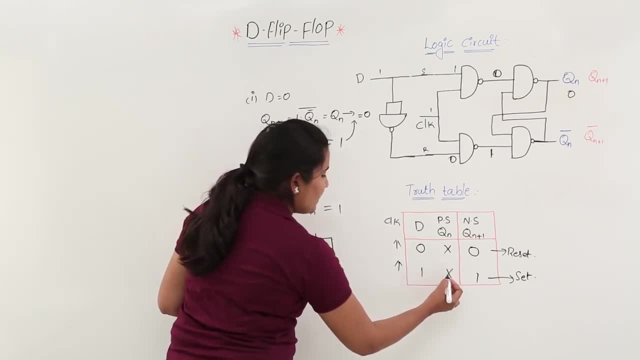 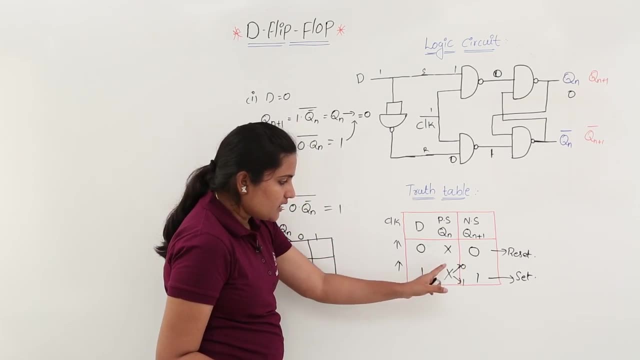 mean. So I am taking combination with 0, 1 and you are getting, when you are having 1 mean. So here you are having 2 states: 0, 1.. In these 2 cases, when d equal to 1 either, q n is 0, also you. 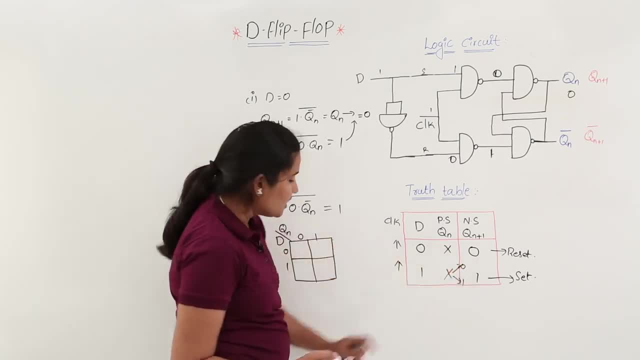 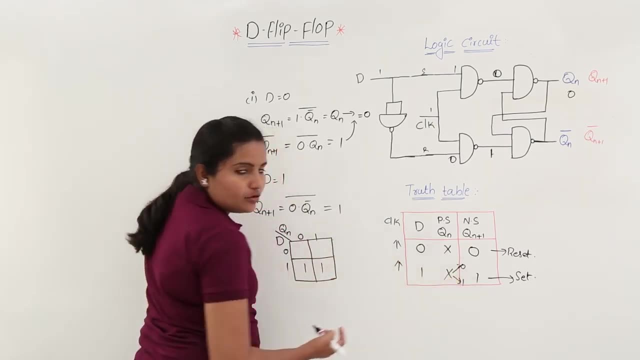 are getting 1 either. q n is 1 also you are getting 1.. So that means when d is equal to 1, both cases of q n will provide you 1.. So here I am just grouping like this. So now this prime. 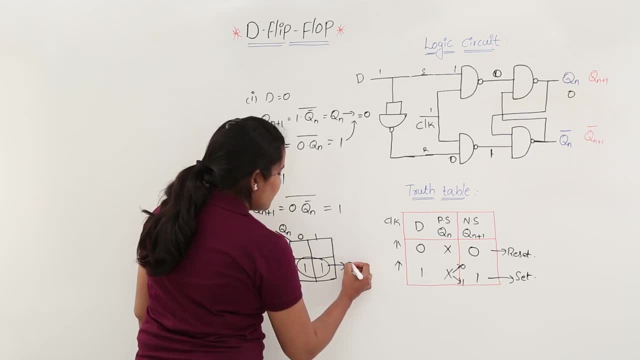 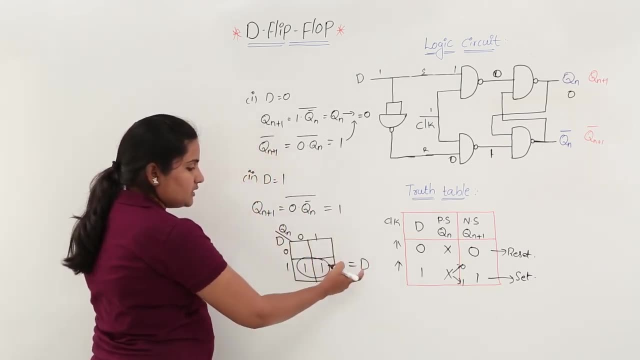 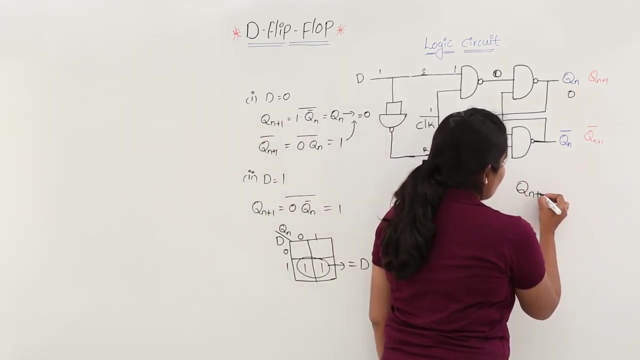 implicant value will provide the equation for a D flip-flop. So sideways it is covering single cell, So D, and here top wise, no combination. this is equal to D. So therefore for D flip-flop, your Q n plus 1 is equivalent to D. So this is the expression for a D flip-flop. So here you. 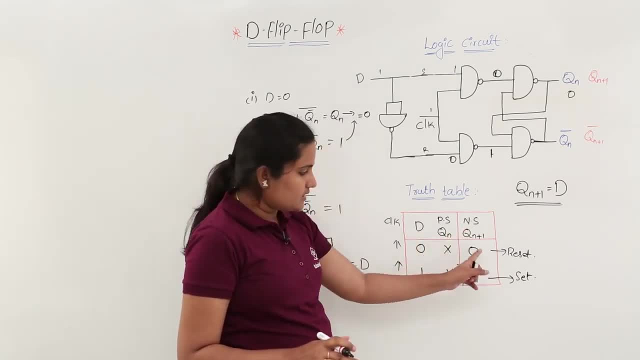 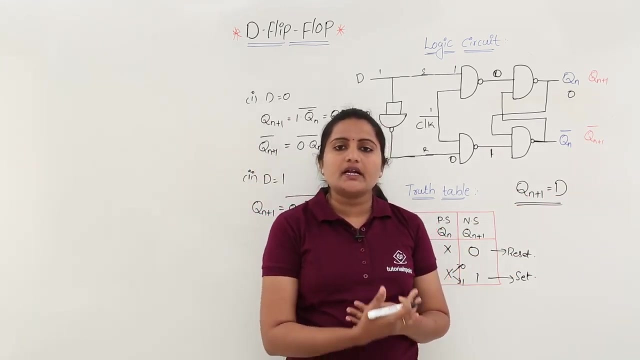 can observe: whatever you are providing at D same thing you are getting at next state. that means output. So if you provided 1, you got 1. when you provided 0, you got 0, same thing we got as expression. this is also called as transparent flip-flop, So that means whatever data available. 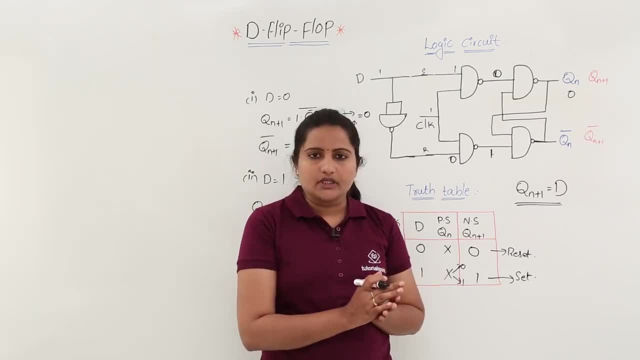 at input. that can be available at output. that is available at output. So that is why this flip-flop, particularly D flip-flop, is also called as transparent flip-flop. So that is why this also called as so data or a transparent flip flop. So here in this D flip flop, just we. 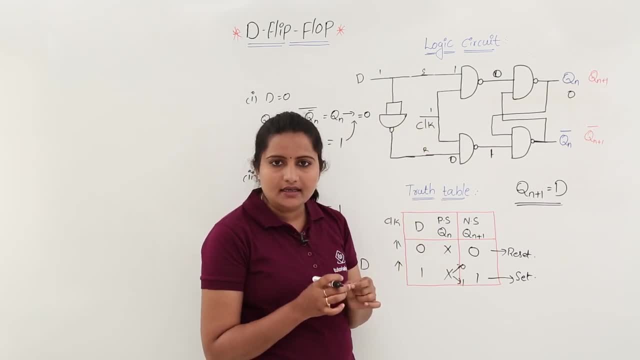 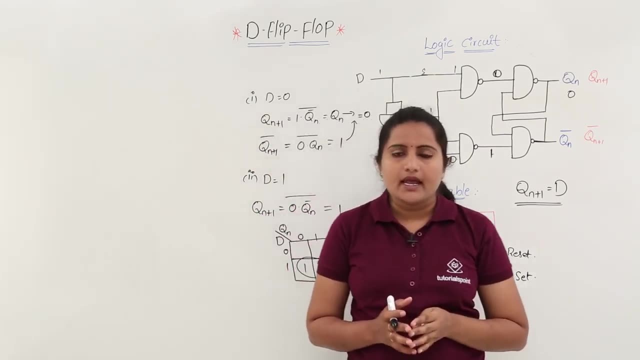 change this circuit. that means we are just adding, we are just clubbing S and R inputs with a, not gate. This is about D flip flop, and in the next class we will design different flip flops like JK and T- all this.